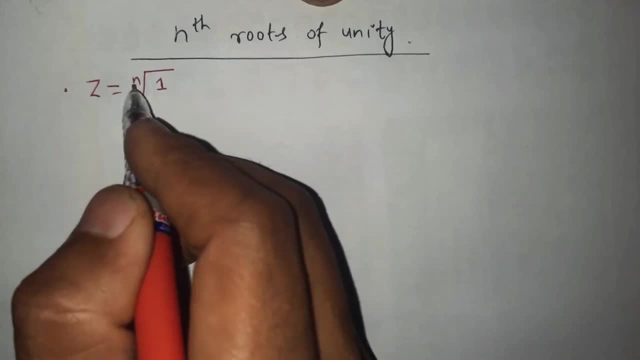 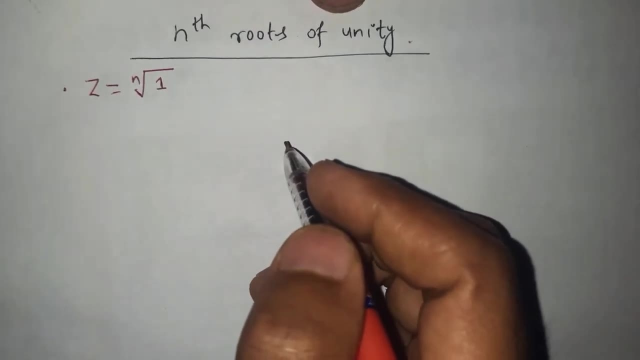 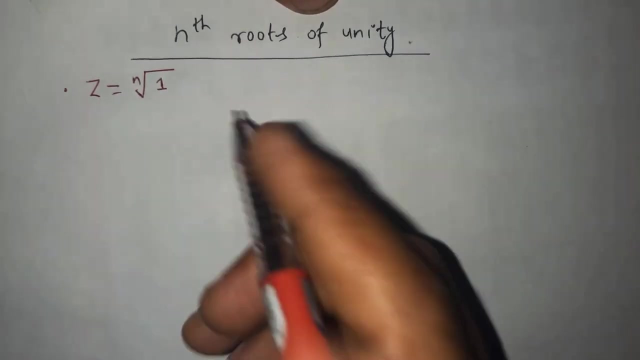 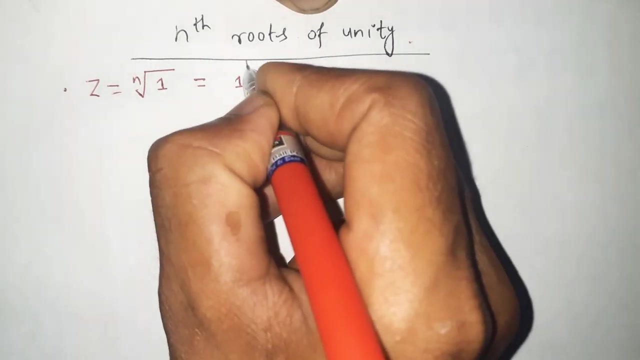 this. This means- here we have written z here- equals to the nth root of unity. Unity means 1.. This is the nth root of the unity. Notation for the nth root of the unity. Let's calculate the possible values of nth root of the unity and this can be further written as 1 to the power of 1. 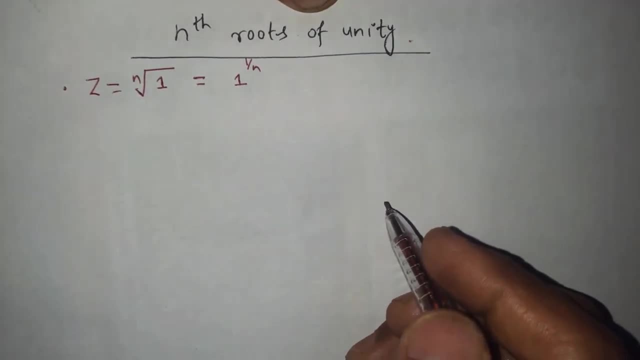 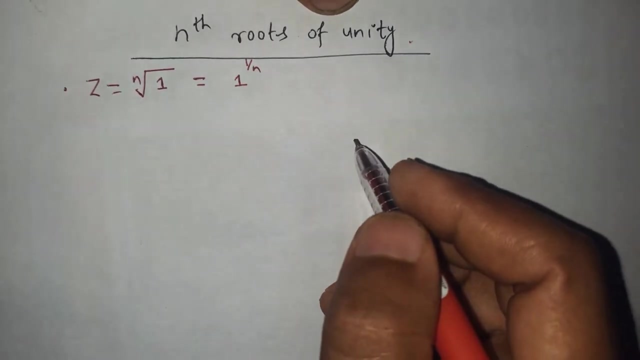 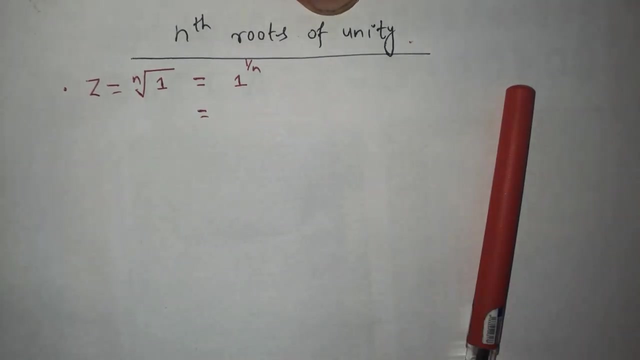 over n. Here we just use the simple property of the indices. We can write this expression in this form: 1 to the power of 1 over n. Just by using the law of the indices. And let's change this 1 in the polar representation, We can change the. 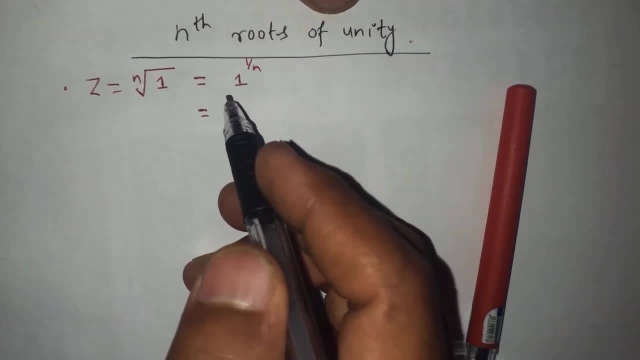 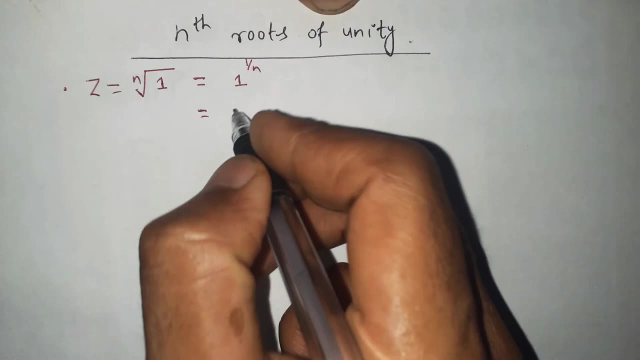 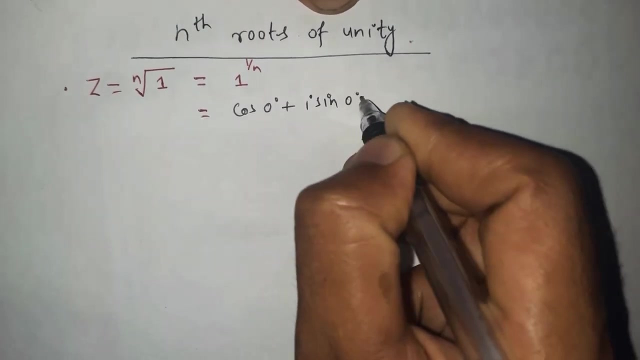 rectangular representation of the complex number into the polar representation. Let's change this 1 into the polar form And the polar form of the 1 is just cos 0 degree plus iota sine 0 degree. This is just the polar representation of 1.. This is just the polar representation of 1.. 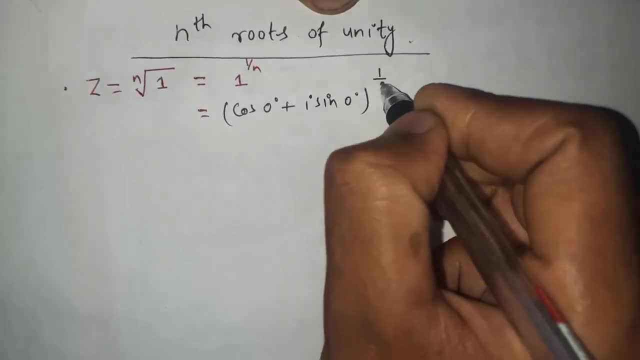 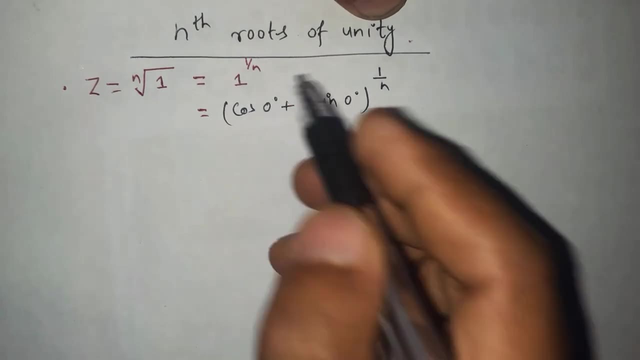 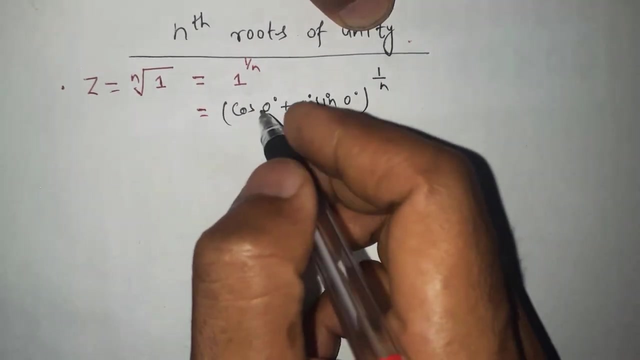 And here it is raised to the power of 1 over n. Here in this second step, we just change the rectangular representation into the polar form. This is the ordinary simple polar representation. Let's convert this simple polar form into the generalization form, And this can be further. 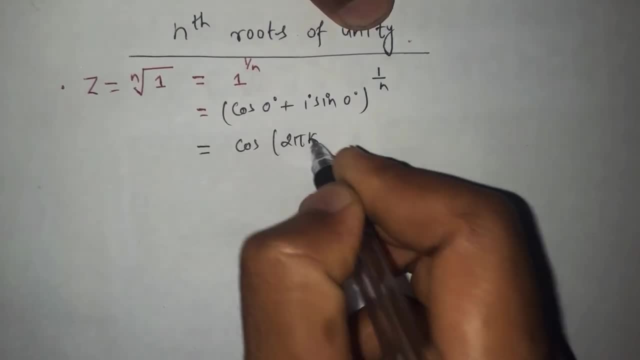 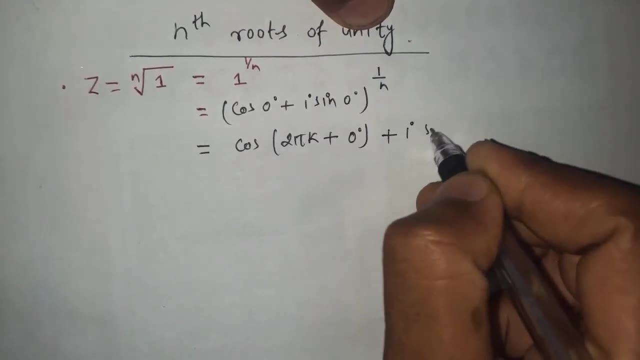 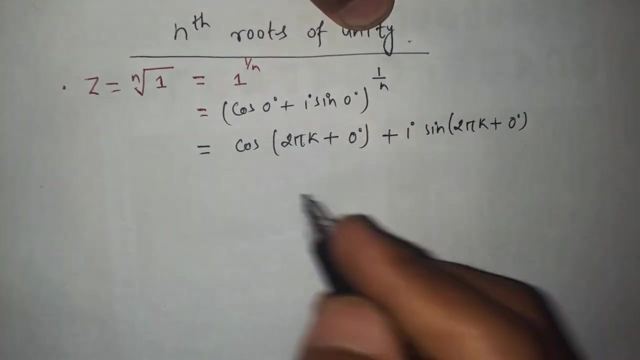 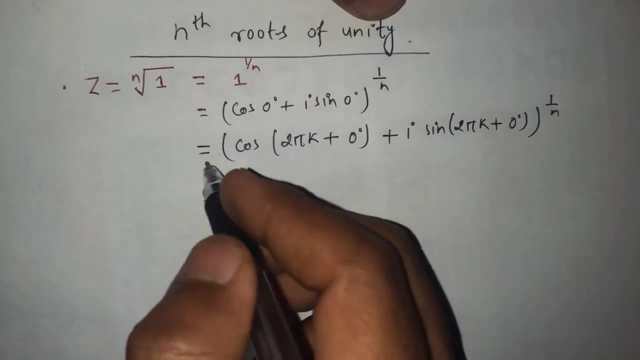 written as cos 2 pi k plus. here the angle is: argument is 0 degree, 0 degree plus iota sine 2 pi k plus the argument 0 degree, And it is here all raised to the power of 1 over n. Here in this third step we 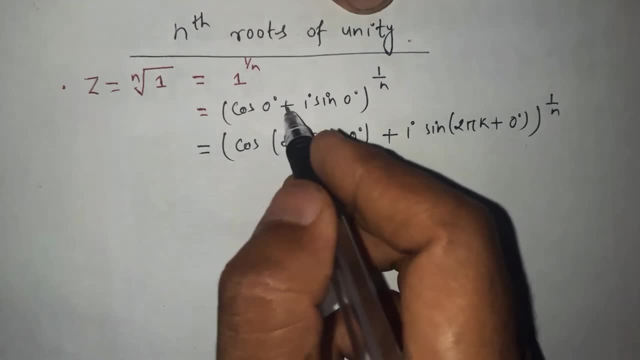 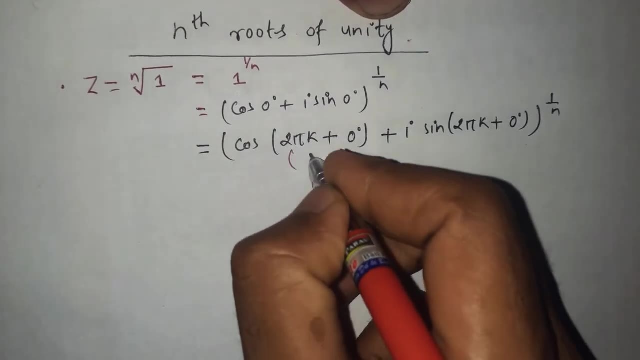 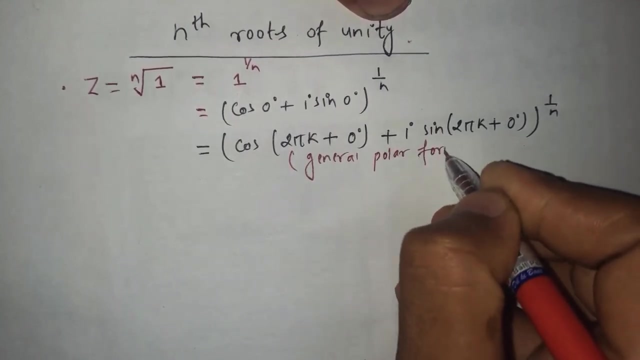 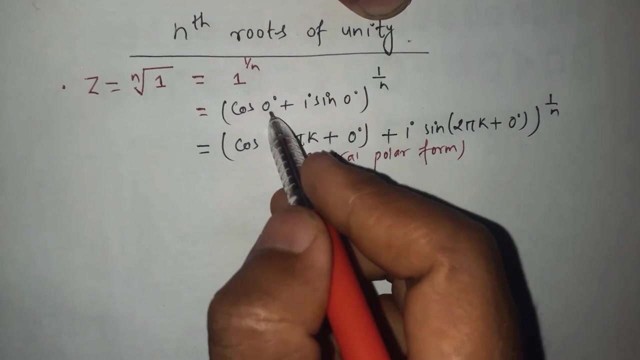 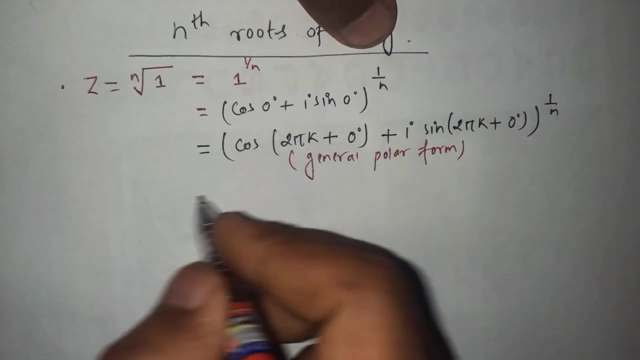 we just change this polar form into the general polar form. This is called as general polar form And this is general polar form. For generalization of the polar form, we have to write, we have to add the argument with 2, pi, k. k is the number which ranges from the 0 to n minus 1.. Where the value of the 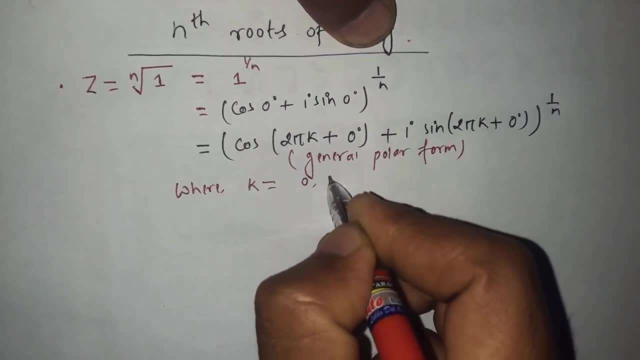 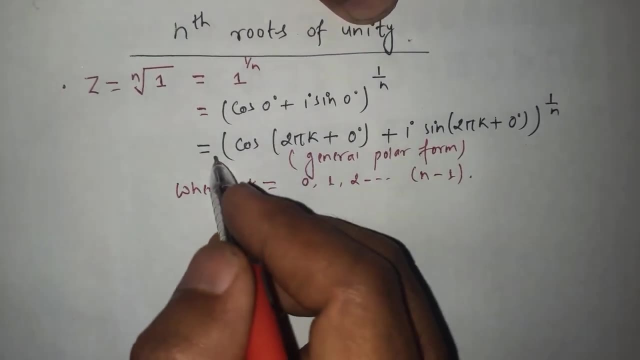 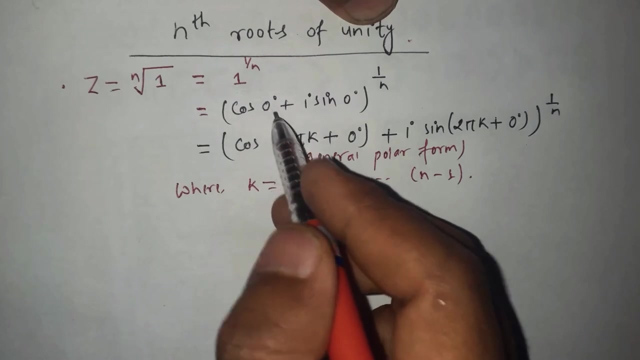 k ranges from 0,, 1,, 2 to n minus 1.. So this is general polar form And this is general polar form Here, in this step. we have just written, we have just written the ordinary polar form into the general polar form. 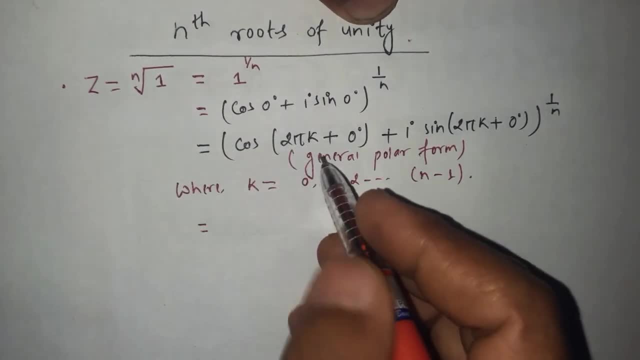 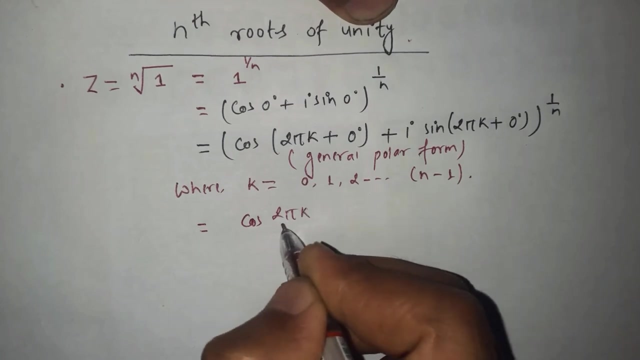 And let's do the further simplifications Here. we can use the Demoravius theorem in this step, And this can be further written as: cosine of this is 2 pi k plus 0 to n minus 1.. 2 pi k plus 0 degree, just 2 pi k. 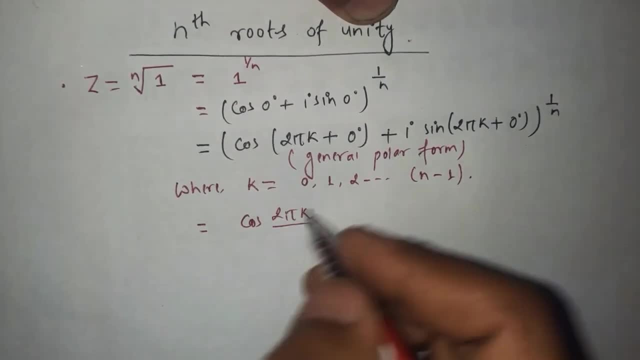 And it is divided by the. it is divided by this number: n over n plus iota, sine 2 pi k, 2 pi k, 2 pi k plus 0 degree, 2 pi k over n. Here we just use the Demoravius theorem on the complex number. 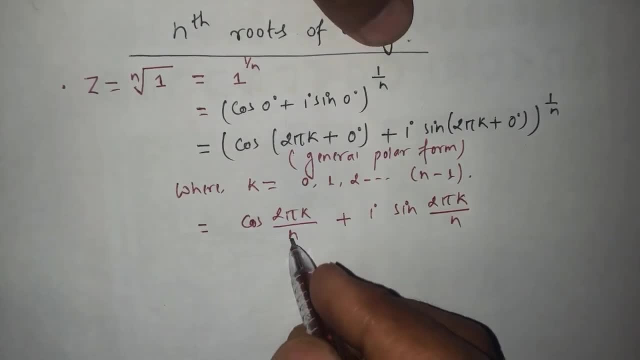 And then let's take the second step. Let's take the third step. Let's take: let's choose the values of the k from 0 to n minus 1, 1 at a time. This is the value of the z. 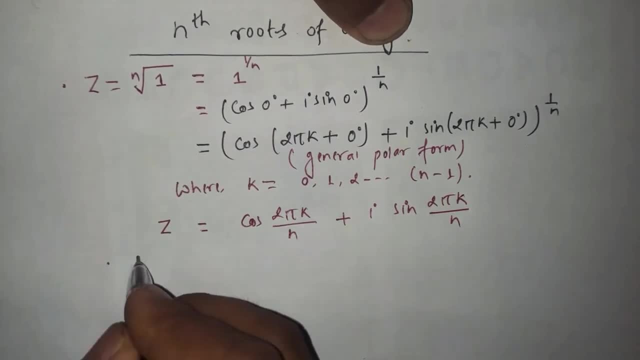 Let's take in the first step. let's take the value of the k. k is a first number, 0, first integer, 0. And this can be. let's write this in the Euler representation, Euler representation form. This can be this: 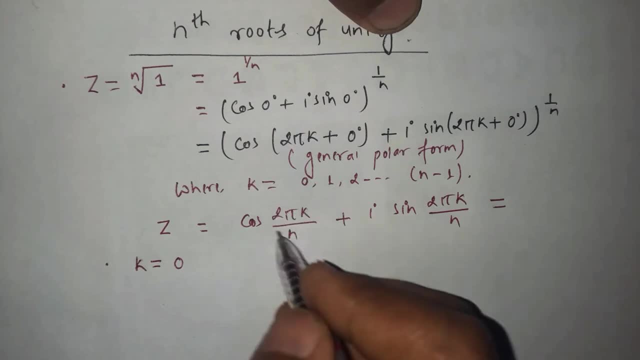 This trigonometric form can be written into the exponential form as the by Euler notation e to the power of i and the angle Angle is here. The argument is this one: 2 pi k over n. Here we have just written into into the exponential form by the Euler notation. 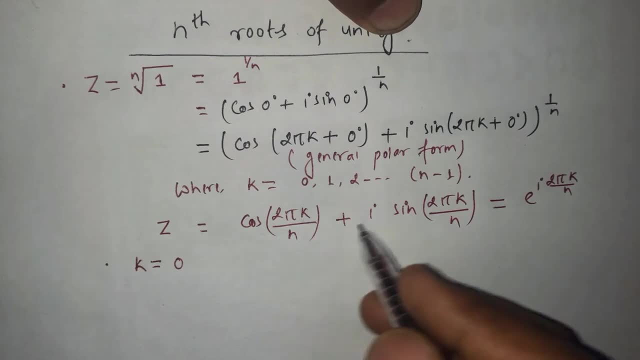 This is the called as the Euler notation. Here we just change the trigonometric form. We just change the trigonometric representation into the exponential. exponential representation. It is Euler notation. And let's take the value of the k as the first integer: 0.. 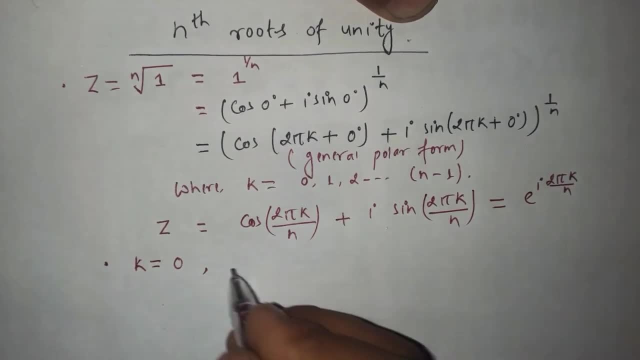 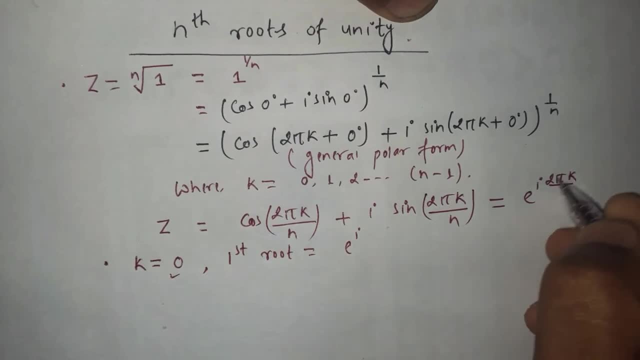 as a 0.. e to the power of this will be the 0.. i times 0. This is just e to the power of 0. And this is just 1.. First root: here. the first root is obtained. here is the 1.. 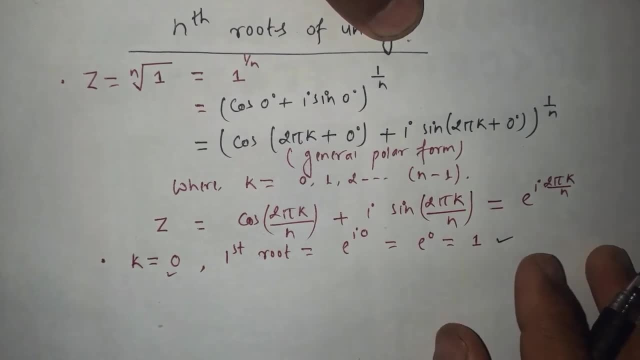 This is the first root of the unity, is the 1.. Let's plug in: the value of the k Is the 1.. And the second root, second root, will be e to the power of here we. we have to just substitute the value of the k by 1.. 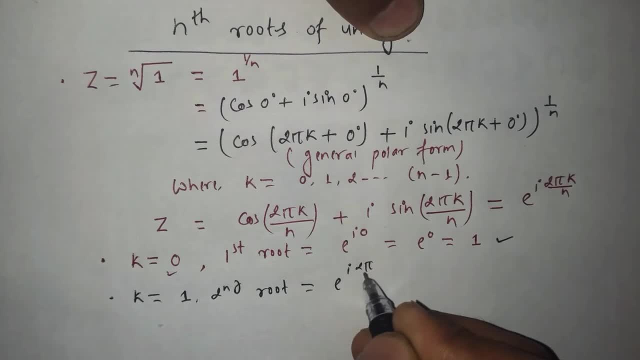 And this will be e to the power of i, 2 pi over n. Here we just substitute the value of the k as a 1.. And let's substitute the value of the k as the 2.. And this will be the third root. 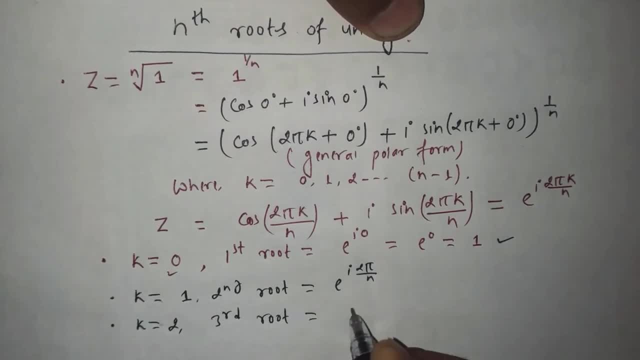 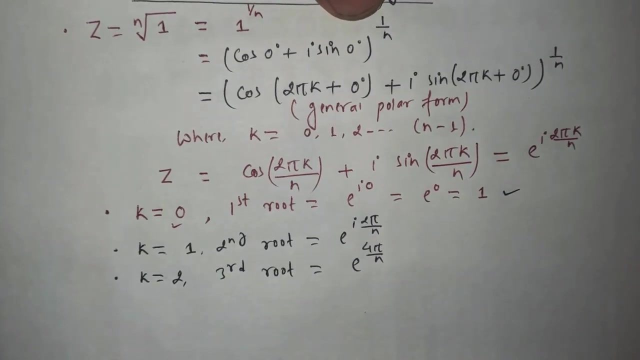 And this is the third root. This is the third root. the third root will be e to the power of. if we plug in the value of the k is the 2, then this will be 4 pi over n. similarly, we can substitute, we can plug in the. 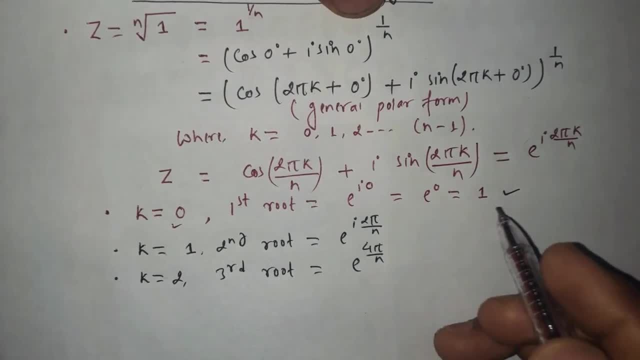 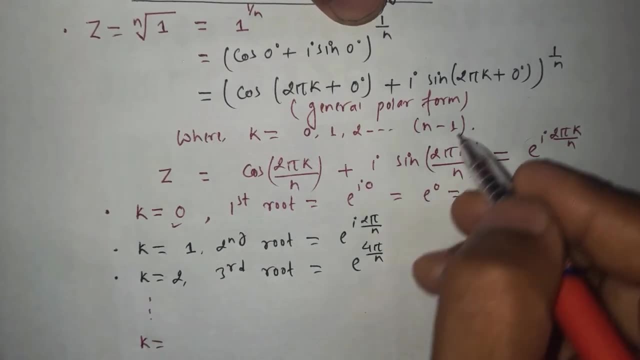 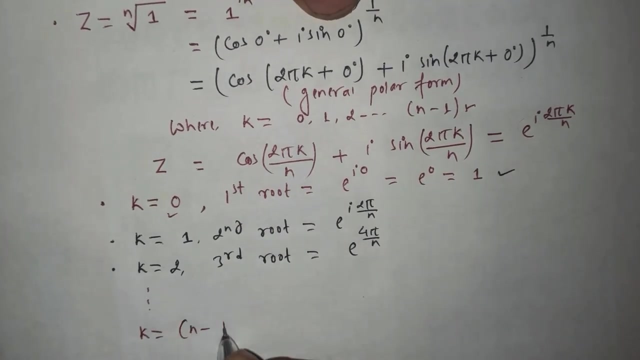 others values of the k in these expressions and so on. if we plug in the value of the k is the last number. is here the n minus 1. k ranges from the 0 to n minus 1. if we plug in the value of the k, is n minus one, n minus one, n the. 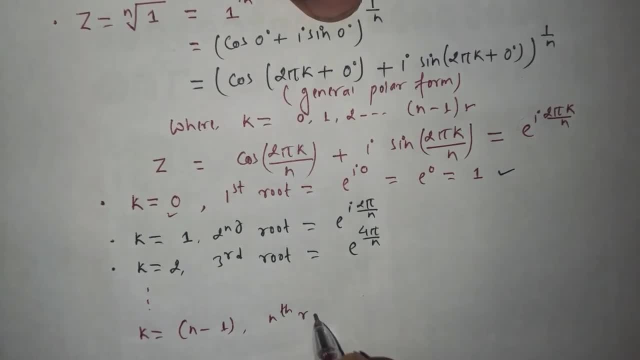 n minus nth root, include. nth root will be e to the power of what will be the value of just a substitute. the value of the k is the n minus one. i to pie, n minus 1 over n, just plug in. the value of the k is the n. 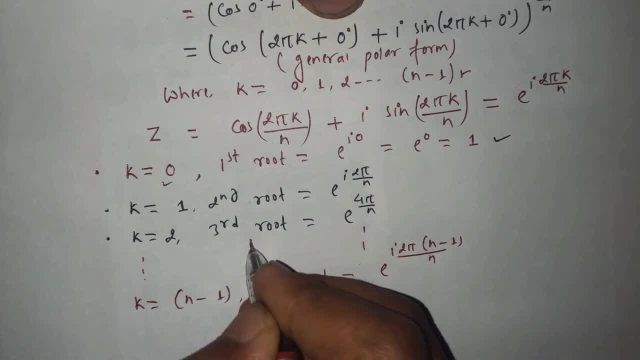 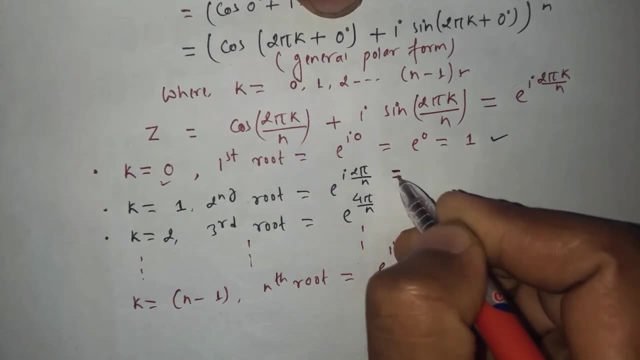 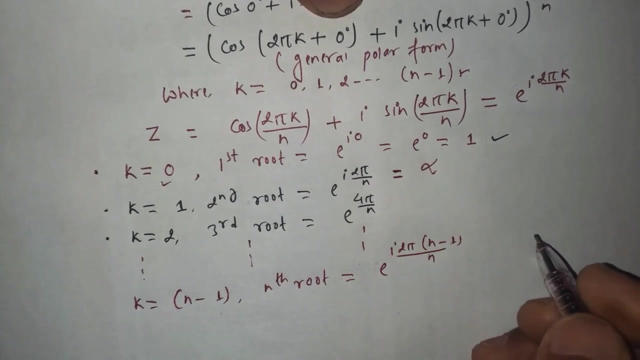 minus one aj. and let's say represent, let's denote this: e to the power of i times 2 pi over n is the alpha. this is the second root. let's denote the second root of the unity is the alpha, and this is just e to the power of 4 pi over n, it is just the. 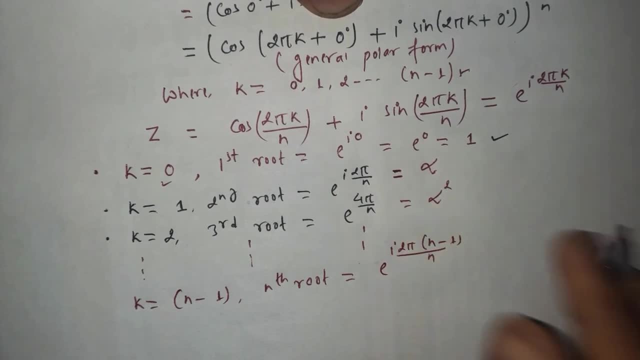 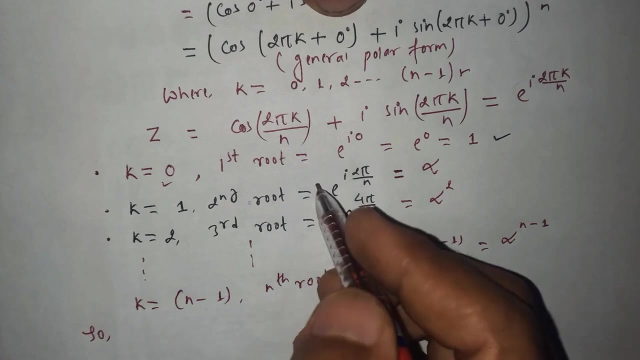 square of alpha, this is just alpha square. if we represent this expression by alpha, then this will be alpha square and this will be just alpha to the power of n minus 1. so finally, we can conclude there. the roots, nth roots of the unity. nth roots of unity are: first: root is 1. the second root is here denoted by the alpha. third, 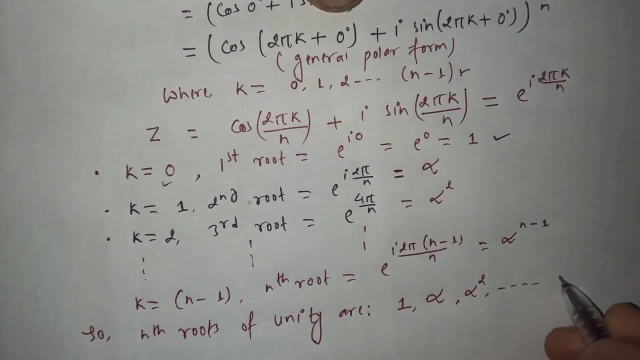 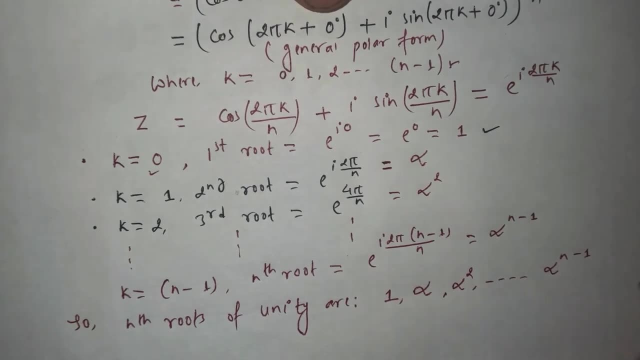 will be the alpha square, and so on up to alpha, to the power of n minus 1. these are the roots of the nth, roots of the unity, where the Greek alphabet alpha represents the a of the root of alpha. so now, from this we can know what is the. 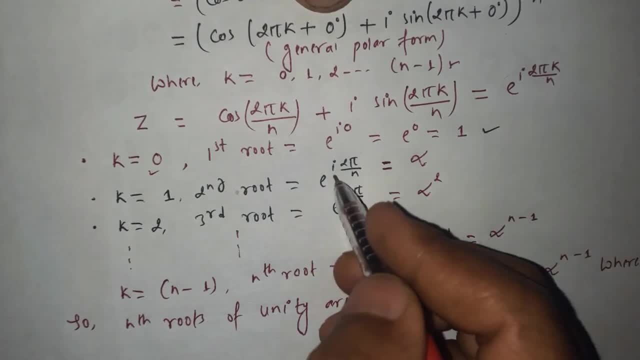 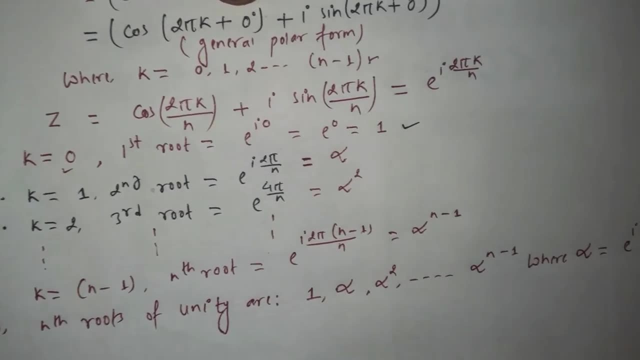 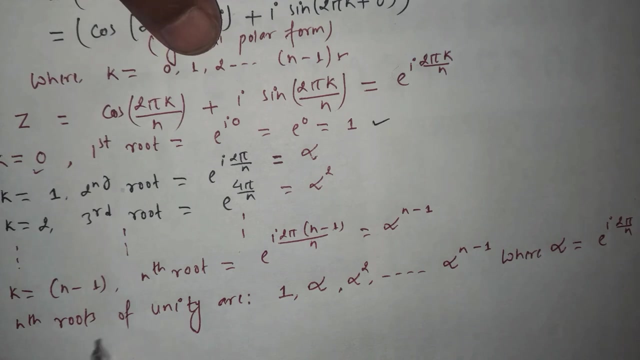 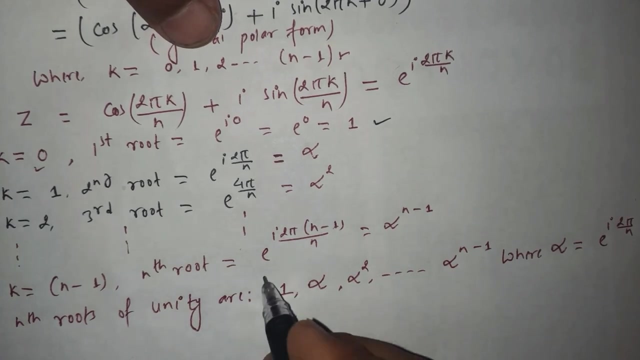 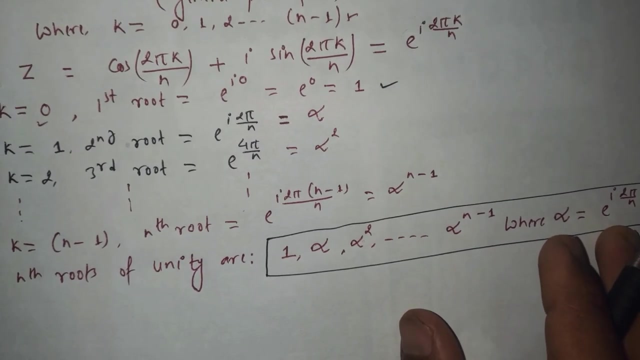 the expression e to the power of i, iota, 2 pi over n. here we have calculated. we have calculated the all the roots, nth roots of the unity. these are the nth roots of the unity. please memorize: these are the nth roots of the unity. let's add the all the nth roots of the unity and let's talk about the one. 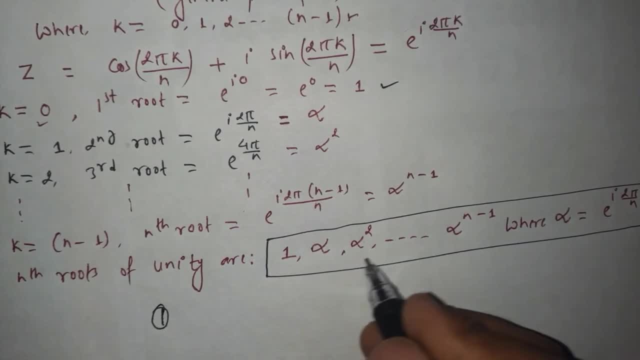 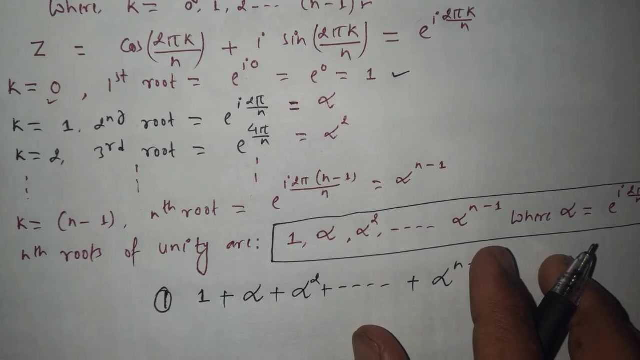 property. let's add all the all the nth roots of the unity. one root is 1 plus, next root is alpha plus, next one is alpha square, and so on, so on, to alpha, to the power of n minus 1. here we just add all the nth roots of the unity and here we 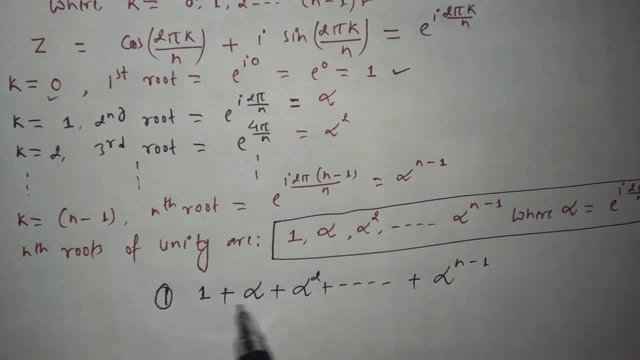 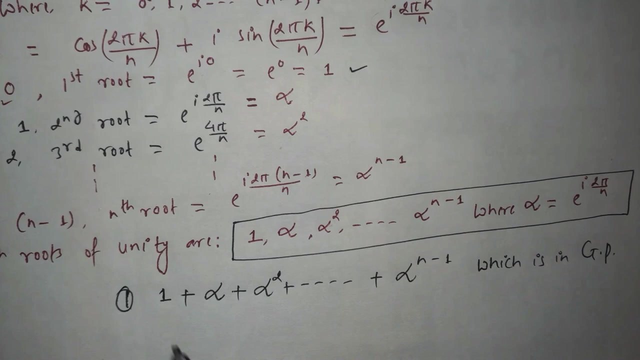 can easily see that these, this series, this series in the geometrical series, which is which is in geometrical progression. here we can easily observe that here the common ratio is alpha. so we can say: this series is in geometrical progression with a common ratio, with common ratio, common ratio. 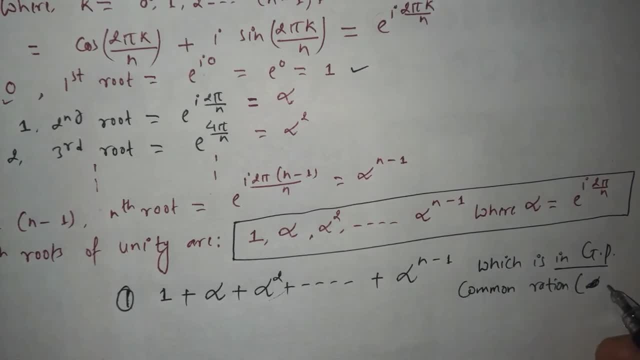 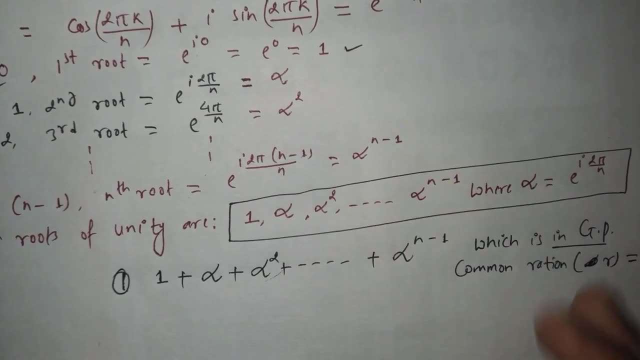 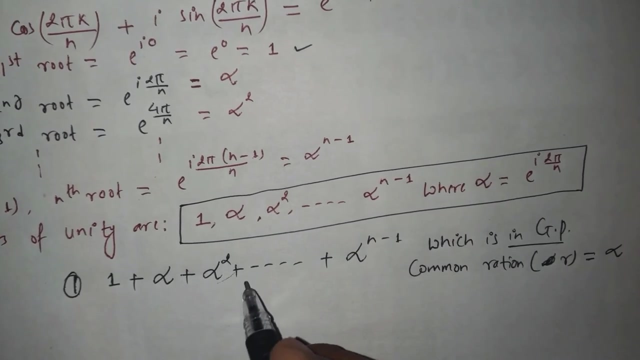 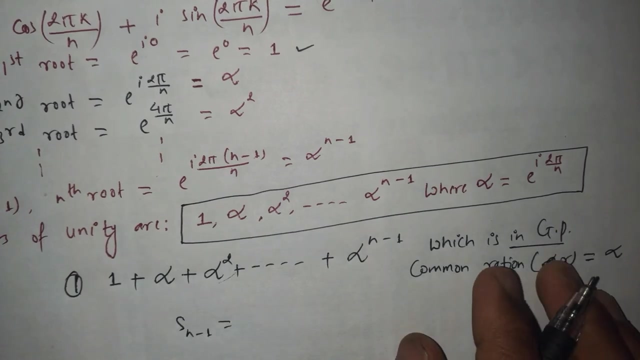 which is generally denoted by the common ratio, is denoted by the R. here it is just alpha. in this series the common ratio is Rety equals to alpha. let's evaluate the sum of the all the terms in the GP: sum some will be some till the n minus 1 comes from 0 to n minus娓a. 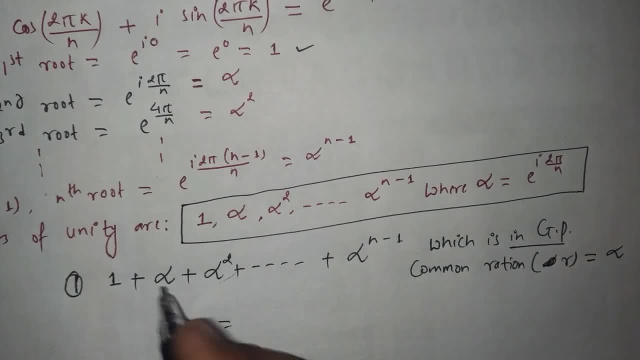 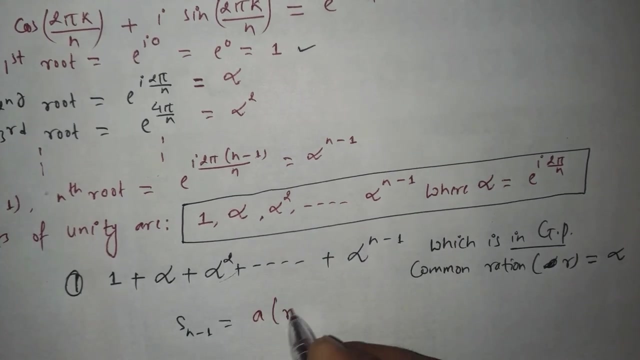 some will be somewhat up to the n minus 1 problems from 0 to m s. one solution, x is, some will be. we have the formula for calculating the sum of the sum of the, all the numbers, all the terms in the gp. we have the formula: a times r to the power of n minus one. 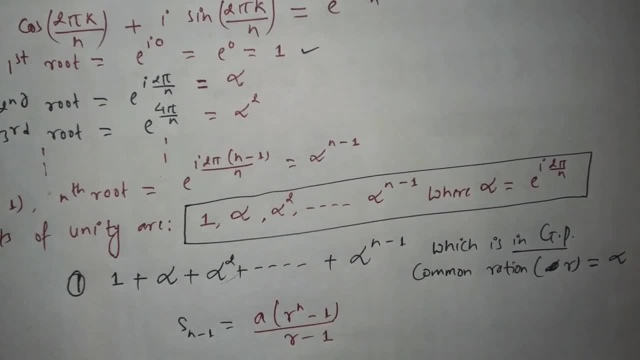 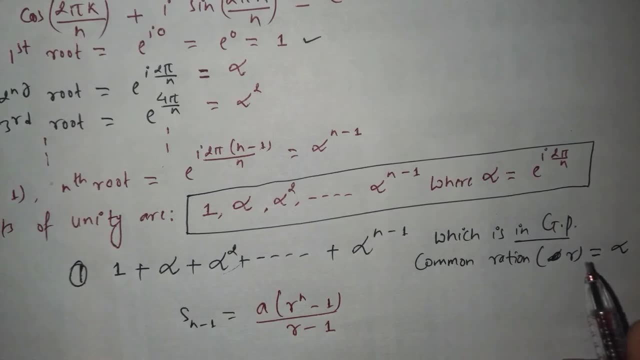 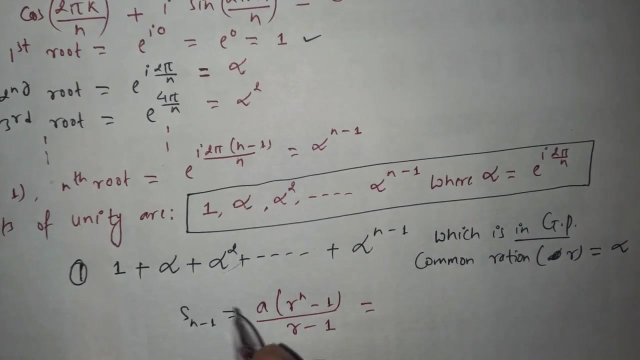 over r minus one. this is the formula uh for calculating the sum of the all the terms in the gp, where r is the common ratio and the a is the first term. let's plug in the value in this formula. here the first term is one, so the value of the a is one. 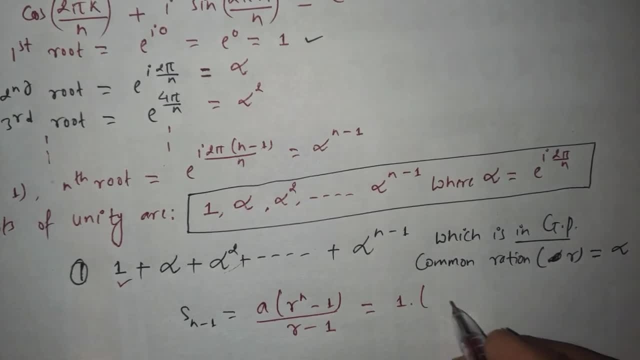 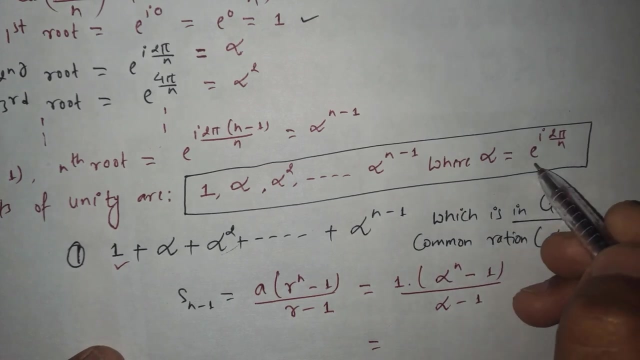 times r is common ratio. common ratio is here alpha, alpha to the power of n minus one divided by r minus one. r is here alpha minus one. and here we have uh, denoted this alpha by this expression: e to the power of uh. iota 2 pi over n. 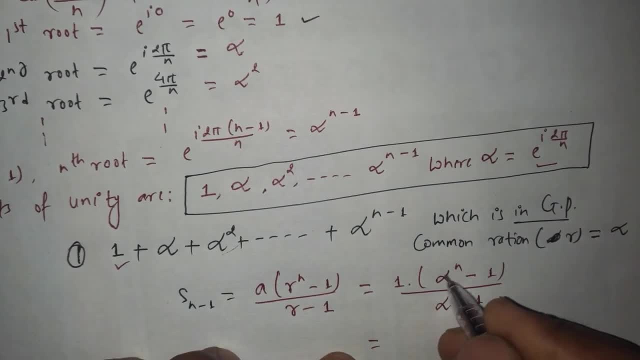 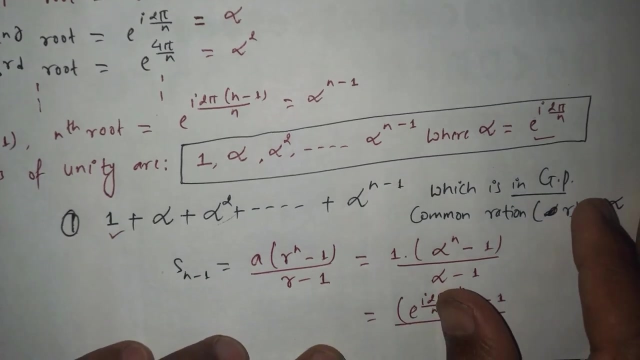 Let's plug in in this expression: and then will be e to the power of i, 2 pi over n. it is all over n minus 1 divided by all, divided by alpha minus 1.. Alpha is e to the power of i, 2 pi over n minus.